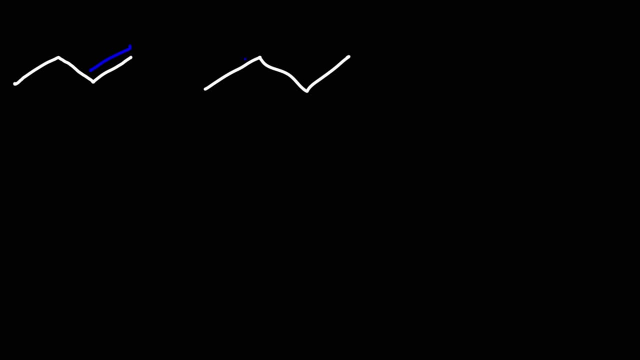 A diene is basically an alkene, but with two double bonds. Now there's different types of dienes. This particular diene is known as a conjugated diene. The reason why it's conjugated is you have alternating double and single bonds. 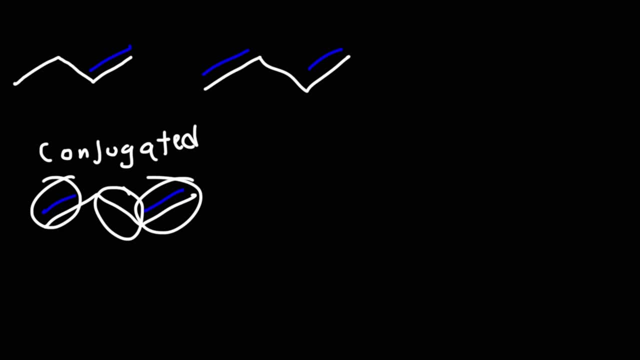 Here it's a double bond. this is a carbon-carbon single bond and that's a double bond. Conjugated dienes have special characteristics. Now there are other types of dienes that you need to be familiar with, So this is an isolated diene. 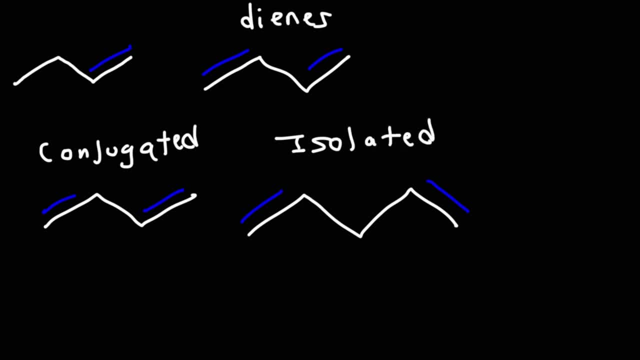 Because? Because the double bonds are too far apart from each other. And then you also have cumulated dienes, So that's where the double bonds are very close to each other. Of these three, the most stable is the conjugated diene due to resonance. 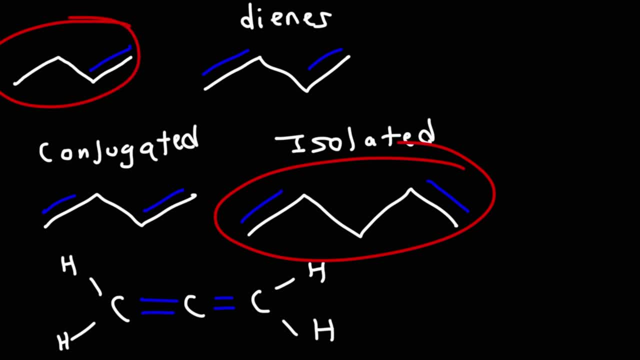 An isolated diene reacts in the same way as a regular alkene, because the double bonds are far apart. But a conjugated diene, It reacts in a different way And we're going to focus on that in our discussion today. So let's begin. 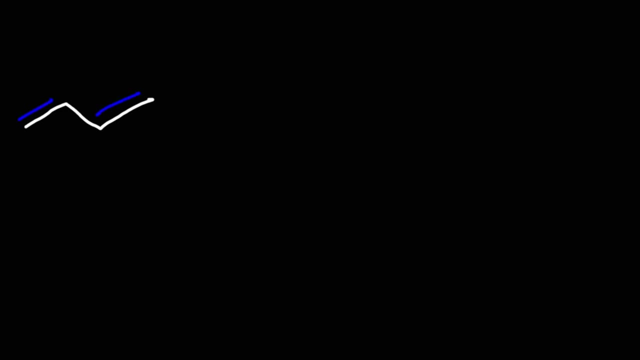 So let's start with this common diene. This is called 1,3-butadiene. If we count the number of carbons, we have a total of four carbons. So think of butane, And we have a double bond on carbon 1 and 3.. 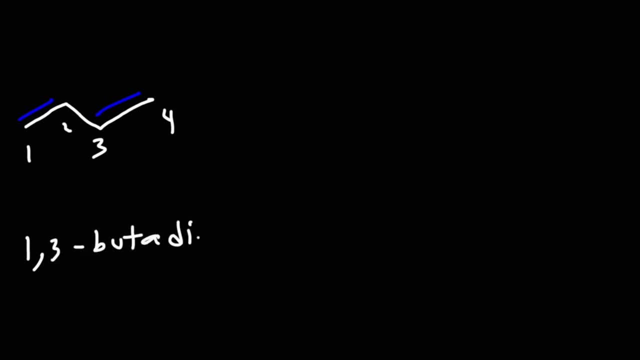 So it's called 1,3-butadiene. Now what we're going to do is we're going to react this diene with hydrobromic acid, HBr, But we're going to react it under two different conditions. 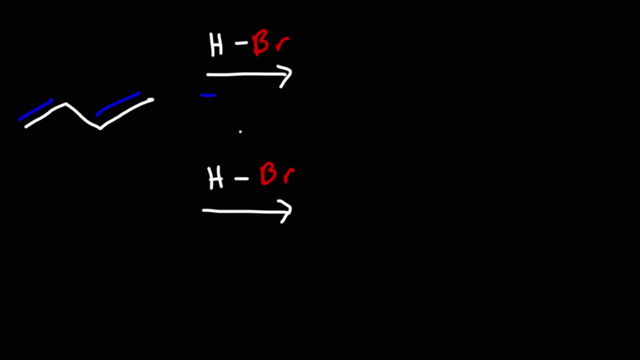 We're going to react it at low temperature, let's say negative 40 degrees Celsius- And at high temperature, which we'll say at 60 degrees Celsius. What would be the major product for this reaction? What would you say? Well, at low temperature, you're going to get something called the kinetic product. 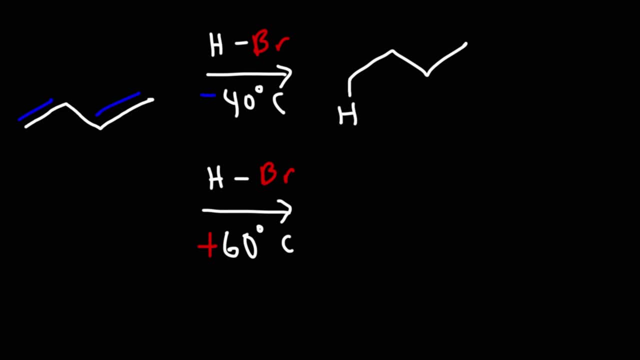 The hydrogen is going to add on carbon 1.. Let's call this carbon 1,, 2,, 3, and 4.. By the way, due to the symmetry of this diene, these two alkenes are equally reactive. 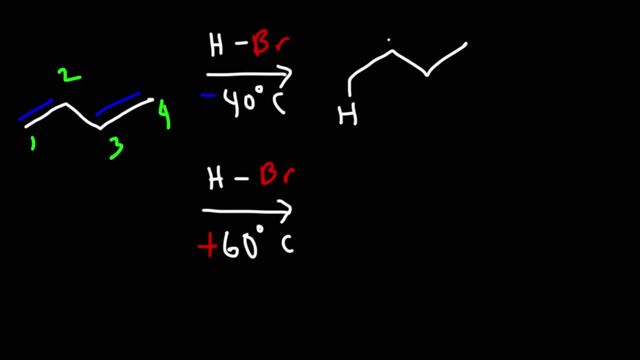 So we're going to react this. So the hydrogen is going to go on carbon 1.. The bromine is going to go on carbon 2. And we're going to have a double bond between 3 and 4.. So this is called the 1,2-addition product. 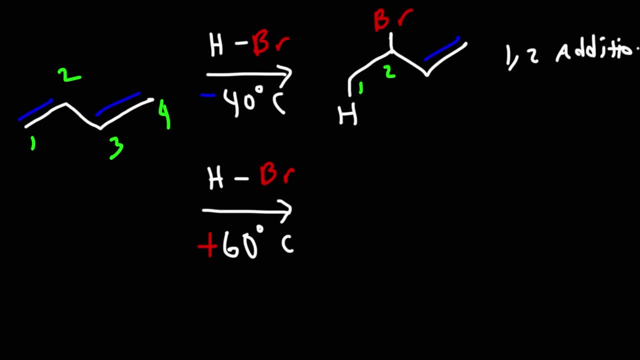 Because HBr added to carbons 1 and 2. Now this is also called the kinetic product, Because it forms faster. Now at high temperatures, the thermodynamic product will be the most stable product. It's going to be the major product. 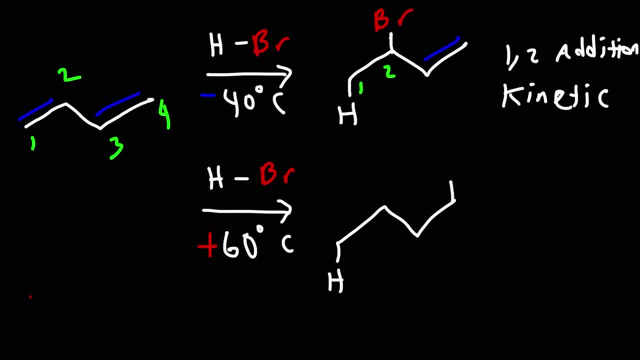 The hydrogen is going to add to carbon 1.. But the bromine atom is going to add to carbon 4. And we're going to have the double bond between carbons 2 and 3. So this is called the 1,4-addition product. 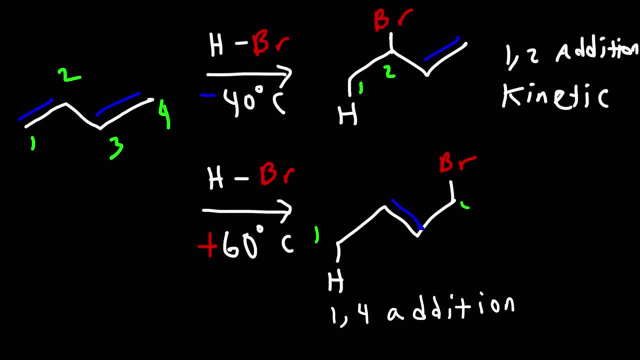 As you can see, on carbon 1, we have the hydrogen And on carbon 4, we have the bromine atom. Now this is called the 1,4-addition product. This is also called the thermodynamic product. It is the product with the most stable alkane. 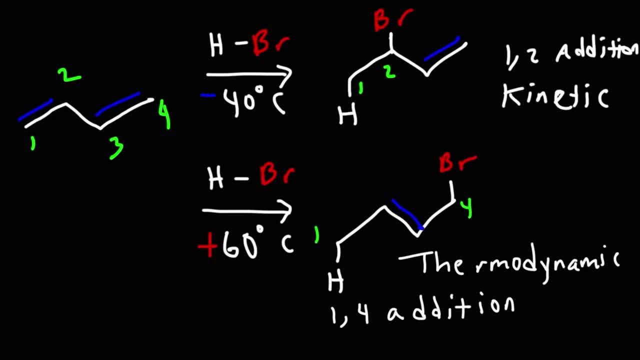 I mean the most stable alkane. I take that back. So this is the product that forms at high temperature. Now the kinetic product. the reaction associated with the kinetic product is an irreversible reaction, So we're going to use one arrow to represent it. 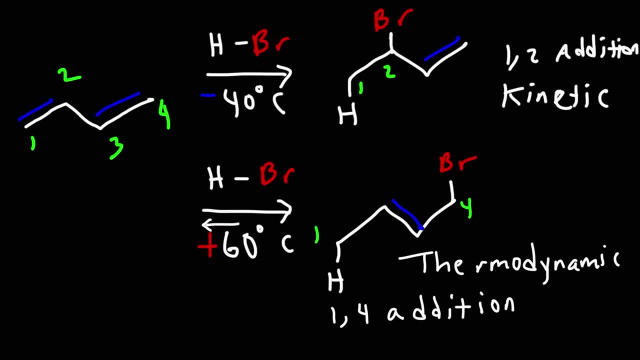 The reaction is going to be 1,2-addition And the reaction associated with the thermodynamic product is reversible. So we're going to have two arrows, But typically the one pointing to the right is going to be the bigger arrow, because this product is the most stable product. 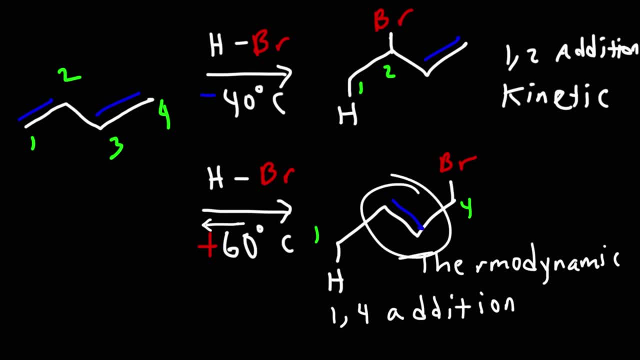 Now let's talk about why this product is the most stable product. The answer has to do with the alkane stability. Notice the number of R-groups that are attached to this alkane. This particular alkane has two R-groups, So it's a di-substituted alkane. 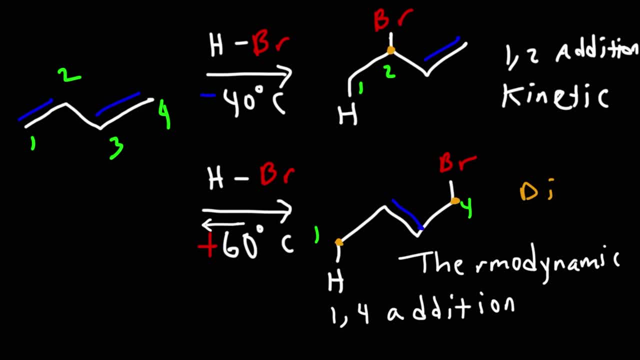 This alkane only has one R-group that are attached to the two carbon atoms that are double bonded. So this is a mono-substituted alkane. So it is the least stable of the two. So make sure you understand that difference. The kinetic product is the product that forms faster. 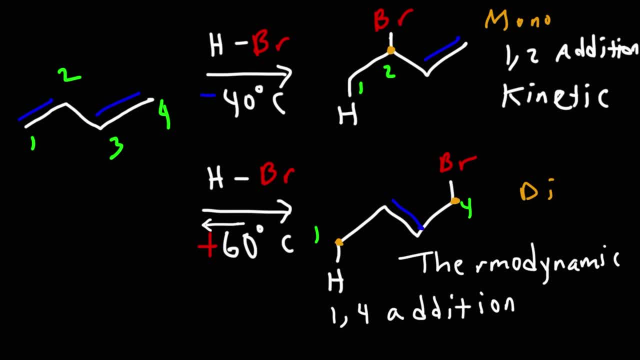 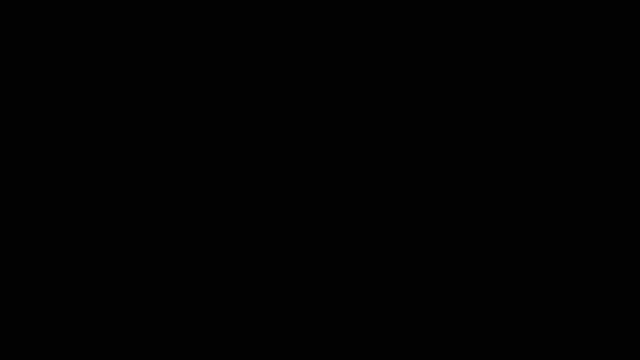 ideally at low temperatures. The thermodynamic product is the most stable alkane product that forms as the major product of the alkane At high temperatures. Now let's briefly review alkane stability. So this is a tetra-substituted alkane. 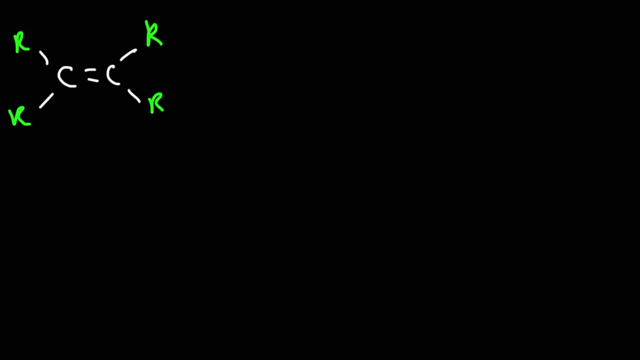 It has four alkyl groups attached to the two carbon atoms that are double bonded. This is a tri-substituted alkane. It has three R-groups: This is a tri-substituted alkane. A tri-substituted alkane is a tri-substituted alkane. 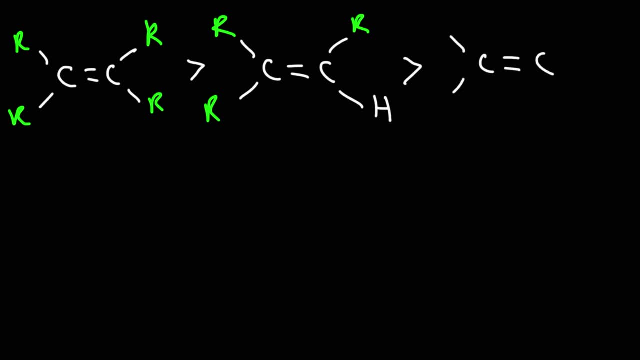 A tri-substituted alkane is a tri-substituted alkane. An alkene is more stable than a di-substituted alkane. Here we have a trans di-substituted alkane And that's usually more stable than a cis di-substituted alkane. 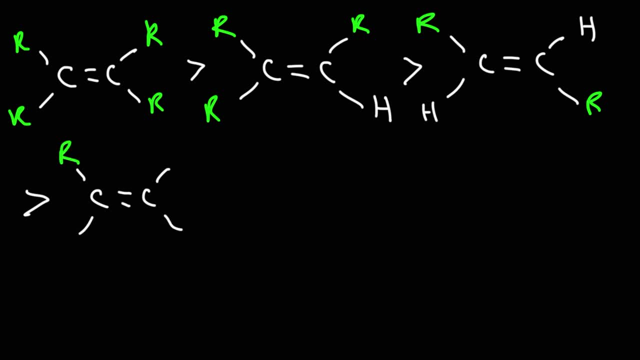 And here we have a mono-substituted alkane which is more stable than ethene, which I'm just going to write like that. So the more R-groups that you have around an alkane, the more stable it is, and that's going to help you to identify the thermodynamic product. but now let's go back to the reaction of 1,3-butadiene with HBr, and this time let's talk about the mechanism. so let's react 1,3-butadiene with HBr at low temperature conditions. so, as was mentioned before, we're going to get the kinetic product as the major product. 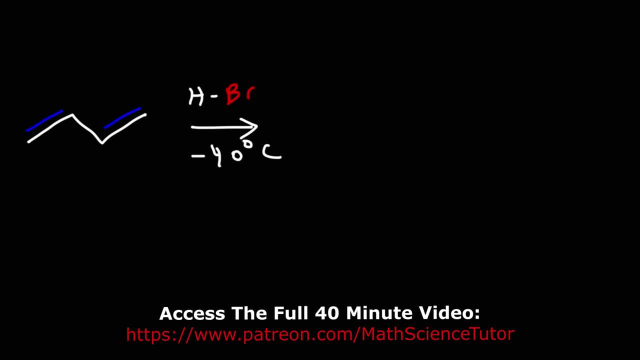 even though both products can form. this reaction is under kinetic control, so the one that forms faster is going to be the major product when its temperature is low. now, in this reaction, the dyene is going to behave as the nucleophile HBr, the acid is going to be the electrophile. 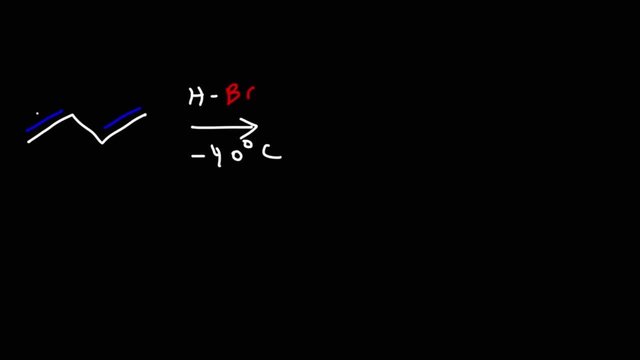 so we're going to write up a mechanism and to show the arrow. just remember when, when drawing the arrow, it's going to start: from a region of high electron density to a region of low electron density. this double bond is electron rich. hydrogen, being partially positive, is electron poor. so the arrow basically describes the direction of 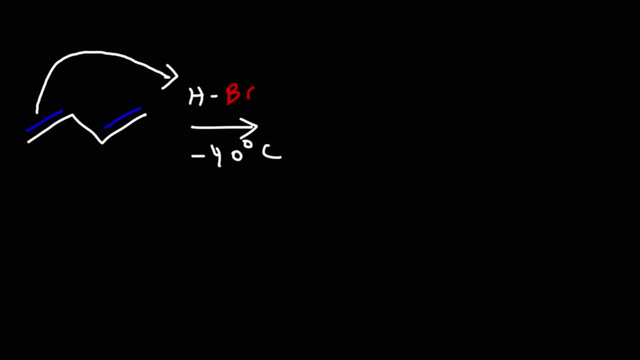 electron flow, so to speak. so when the double bond interacts with the hydrogen, the bond between HBR is going to break. those two electrons is going to be pulled towards the more electronegative bromine atom. now here's a question for you: why should we put the hydrogen on carbon 1 and not on carbon 2? notice what. 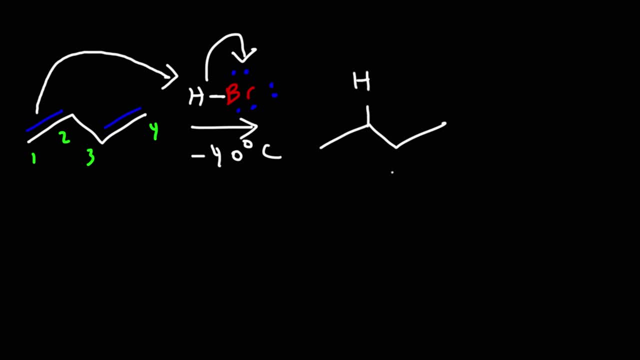 happens if we put the hydrogen on carbon 2. if we were to do that, we would get a primary carbocation, but if we were to put the hydrogen on carbon 1, the plus charge would be negative. so if we put the hydrogen on carbon 1, the plus charge. 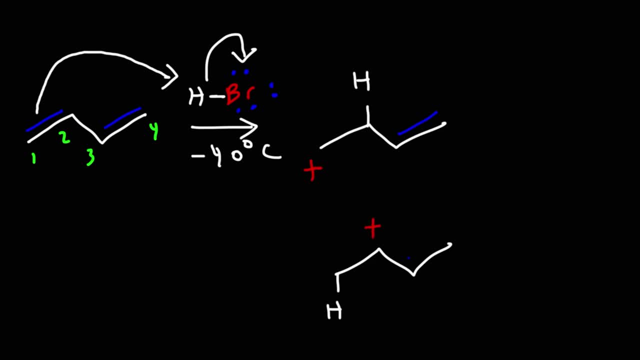 is going to be on carbon 2, so we get a more stable secondary carbocation, but notice that it's adjacent to a double bond. so what we get is a secondary allylic carbocation, and so that's the reason why hydrogen is going to add on. 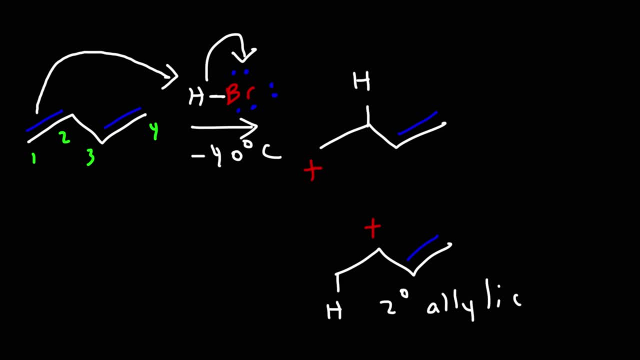 carbon 1. it's because we get a more stable carbocation intermediate. that's the first thing you need to consider. where will the hydrogen go now? what will the bromine atom do, or more specifically, the bromide ion now? by the way, this structure has a resonance structure. we could move the alkene here. 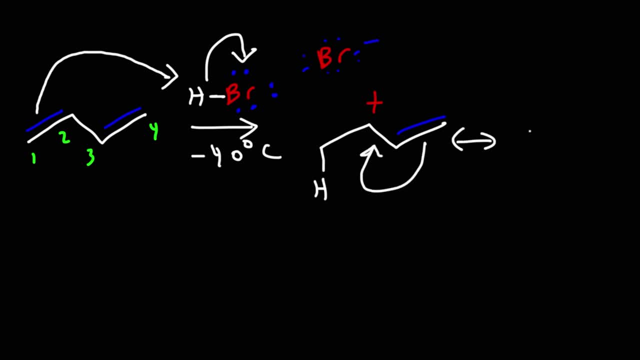 if we take those two pi electrons and move it to the left, we can get another intermediate. so this is going to be a less stable primary allylic carbocation. so this is secondary and this is primary. so just looking at the carbocation stabilities, this particular resonance, 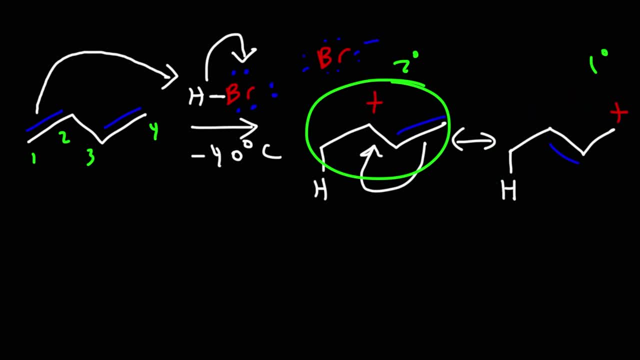 structure is more favorable than this one. so, because the secondary allylic carbocation is more stable, it's going to form faster because there's less energy that's required to generate this particular resonance structure. now, which carbocation will the bromide ion interact with? is it going to be the 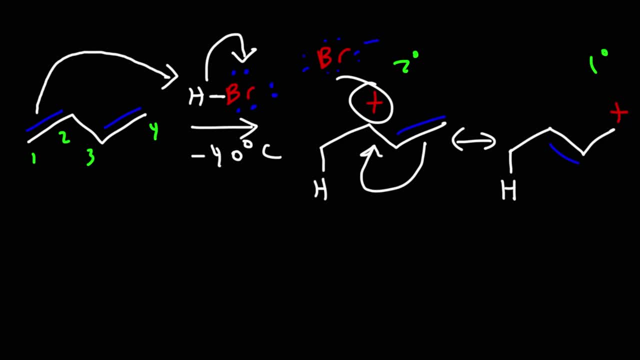 secondary carbocation or the primary allylic carbocation. well, as was mentioned before, the fact that this is more stable means that bromide is more likely to interact with this secondary carbocation. but that is not the only reason. there's also something called the proximity effect. 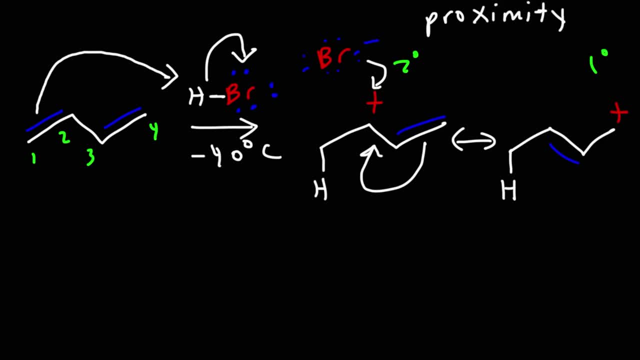 because bromide is so much closer to the secondary carbocation, it's easier for it to interact with that particular carbocation. this positive charge is further away from the bromide ion, so it's less likely that the bromide ion is going to interact with the primary carbocation. so therefore there are two. 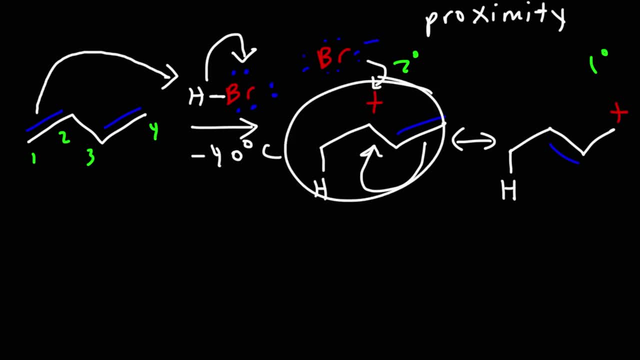 factors that are favoring the one two kinetic product. the first most important factor is the proximity effect and for this specific example, the second thing is we have a more stable carbocation intermediate. so once the bromide ion combined with the carbocation, we're going to get the one. 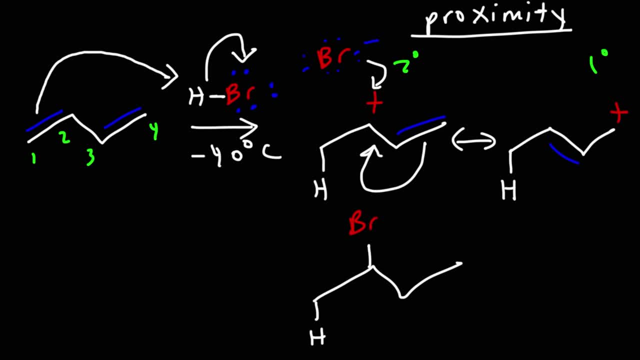 two addition product. so at low temperature conditions this is going to be the major product and the driving force is the proximity effect and the fact that we get a more stable carbocation intermediate. now let's draw the resonance structure for the formation of the one four product. so let's react one three butadiene with 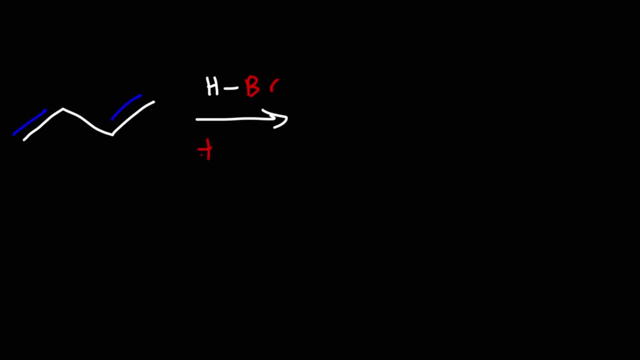 hydrobromic acid at high temperature conditions. so let's use positive 80 degrees Celsius. so at a high temperature. this reaction is reversible, so the most stable alkene product will be the major product. so, like before, we're going to react the alkene with HBR. 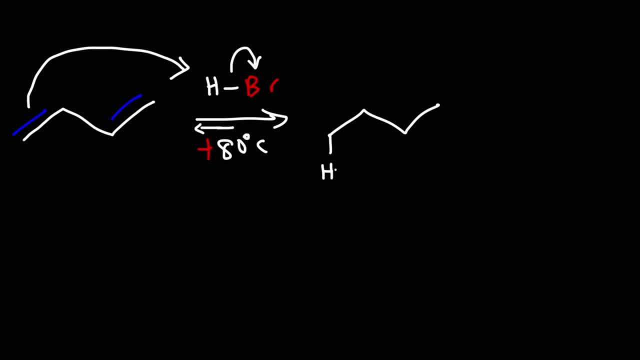 and we're going to put the hydrogen on the primary carbon so that we can put a positive charge on the secondary carbon. now to get the one four product, we need to draw the resonance structure where this double bond is going to move. here and now we have the plus charge on the primary allylic carbocation.